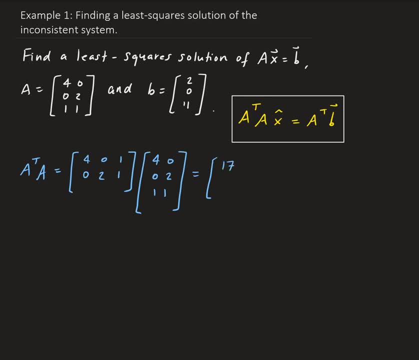 so we're gonna get four times four, sixteen plus one, so that gives us seventeen, and then we have four times zero. that's zero plus zero plus one. and then we're gonna get a c- zero plus zero plus two, a plus- i'm sorry- one, and then zero four and one, so it's going to give us five here. okay, so now we have to. 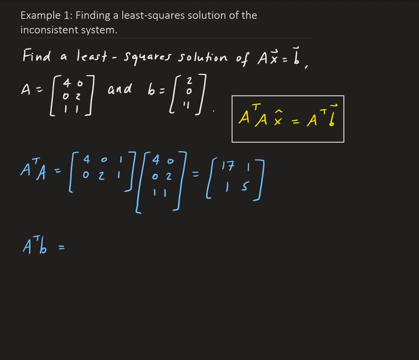 compute a, transpose b. so the four zero one, zero two. one. eight times b: two zero one, one. okay, so this is going to give us a, two by one, so we have eight. so four times two, eight plus eleven, it's going to give us 19.. 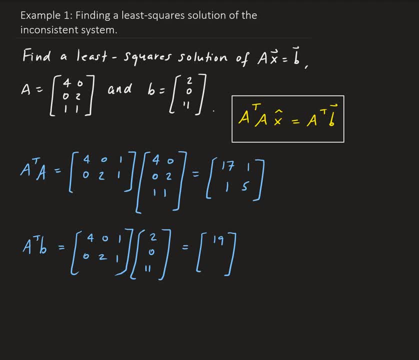 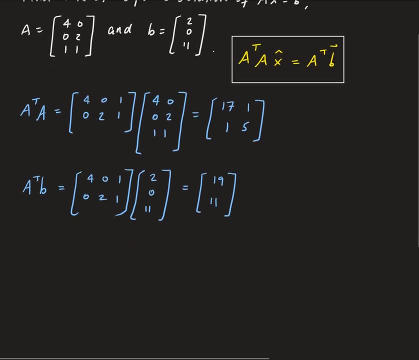 and then we have zero plus zero and then plus eleven, okay, okay. so now our system, right, okay. so we have a transpose a, okay, which is here okay. and then we have a transpose times b, which is here okay. so we have okay, uh, 17, 1, 1 and 5. 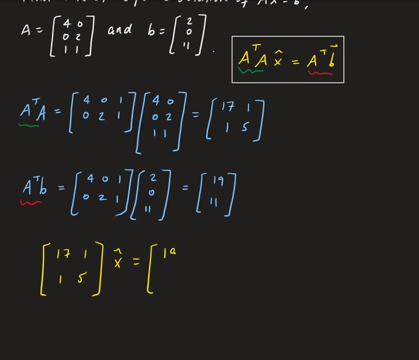 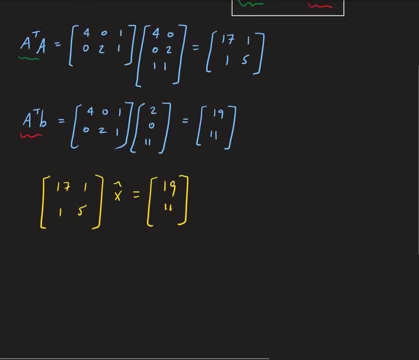 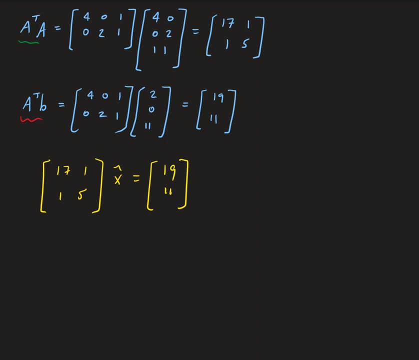 times x, hat equals to 19, 11.. okay, all right, so we can go ahead and we can solve this by taking the transpose- okay- of this matrix here. okay, so, a transpose, a inverse, okay, so we're going to take the inverse of 17, 1, 1 and 5.. 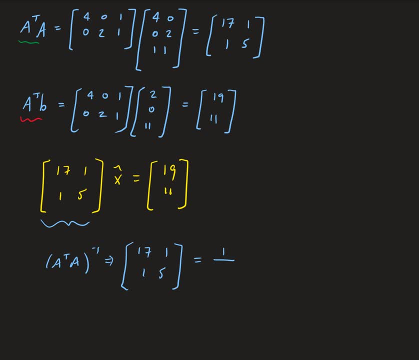 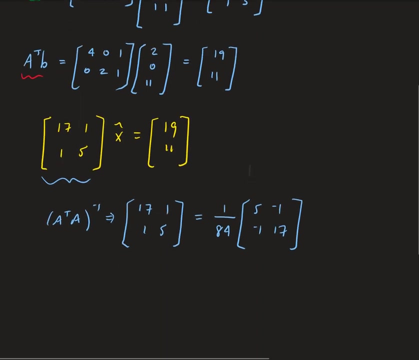 okay, so that's going to be 1 over. the determinant of this matrix is 84. okay, and then we're going to multiply this by the matrix 5 negative, 1, negative 1 and 17.. okay, all right, so we're going to take this and we'll multiply it by our vector 19, 11.. okay. 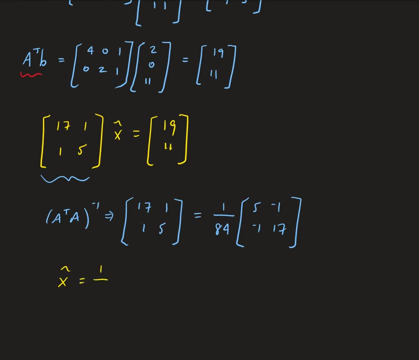 so x hat will be equal to 1 over 84 times 5 negative. 1 negative 1, 17, and then times this vector. so this is going to give us, okay, uh, 1 the vector, 1, 2. okay, all right, so that is our least squares. 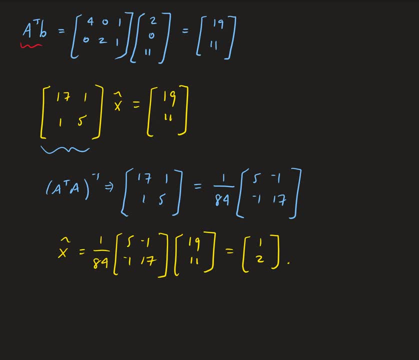 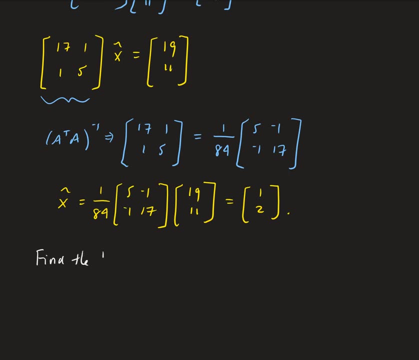 solution. so now let's calculate the least squares error. okay, okay. so the least squares error is going to be right. it's the: the distance between b, between the vector b, and ax hat. so we're going to take the norm. okay, the length of this vector, which is the, which is the norm. 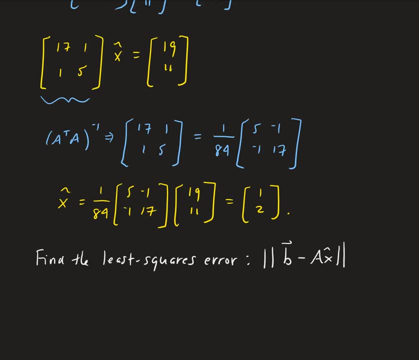 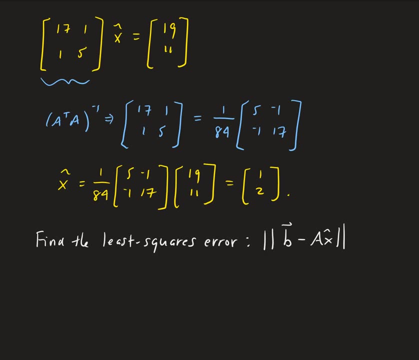 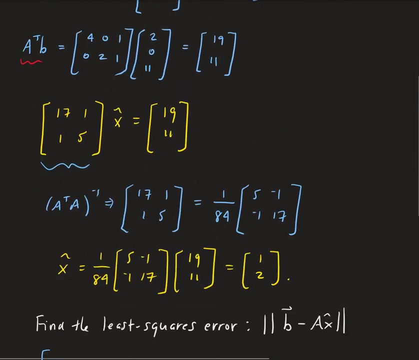 in a letters scratch form that's going to give us data about this vector. okay, all right, so that is so. if your car, if you remember from the previous videos, this is the Z component, so this is right. so this is in the orthogonal complement of the column space of A. okay, all right, so now. okay, so we have. so B was CB, was 2 0, 1, 1 or 2 0, 11. 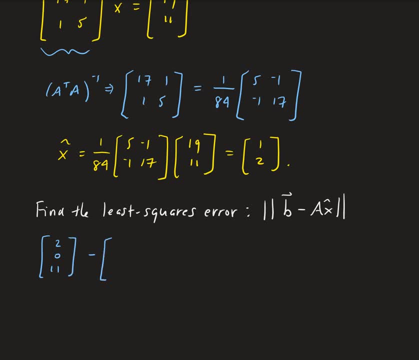 mine. so a was four zero, zero, two, one one times X, just one, two, okay, all right. so this, okay, this is gonna give us: we have two zero one, one minus, okay, so we're gonna get, let's see, four, okay, and then four and then three, okay, all right. so. 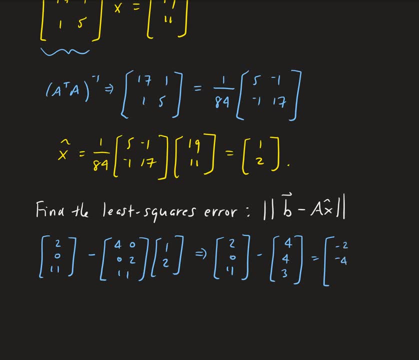 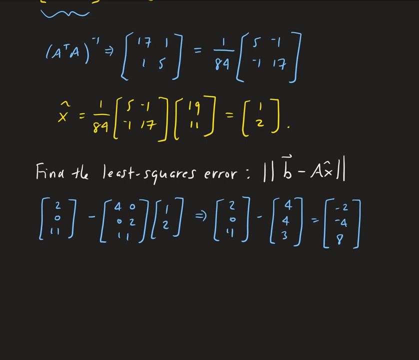 then we have minus two negative four, and let's see nine. okay, oh, sorry, not nine, this is eight, sorry, okay, all right, let's see. just double-check everything here. so, you, you, okay, okay, so now. so now we have the vector, we have the difference of B and 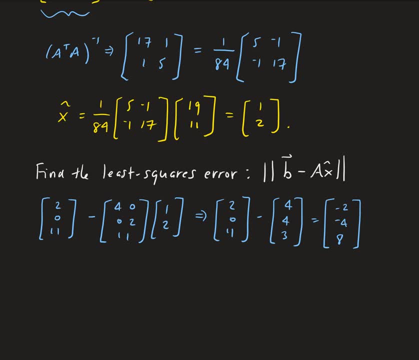 ax. so we're just going to take the right. we need to calculate the length of that, okay. okay, so to get the length, it just basically the length of the vector is just squaring the components, okay, and then taking the square root. so we're going to have minus two squared plus negative four squared, okay. 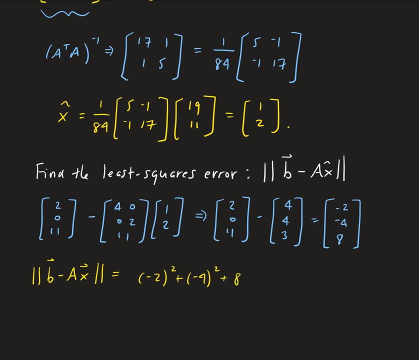 you minus two squared plus eight squared, okay, and then we take the square root. so you, okay, and then taking the square root, so this is uh, so this is what's called the. this is uh, so this is what's called the Iuclidean Norm Meatletter. okay, all right, so let's do a calculation here, so just. 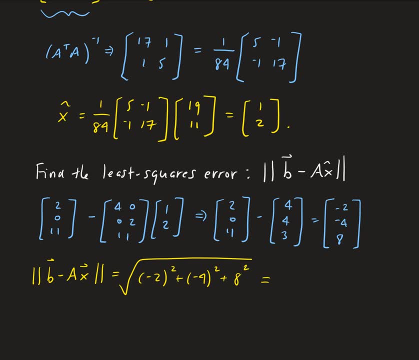 so we have, so we have mais two. Okay, so, yep, so we get square ofWell then let's see multiple. okay, so let's see if we did that. so this is going to be 84. yes, I Вам 그건 84.. 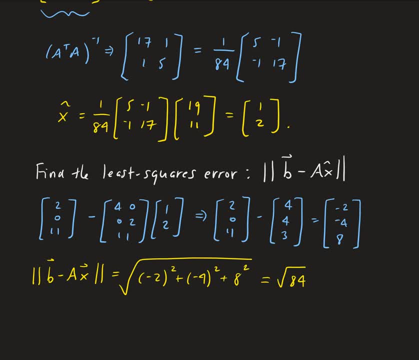 okay, so, yeah, so we get the square root ofArial, So this is going to be 84.. like this, the second derivative of b9. I have times 18: estás en cette term. you can see that there are 13.. and then the square root of that. this is going to be approximately nine points. 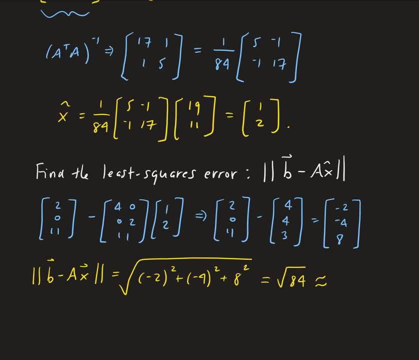 let's round it to two decimal places. so nine point one seven. okay, so that is the least squares error. that's the minimum. okay, that's them. that's the smallest error we can get because of the orthogonal decomposition theorem. okay, all right.